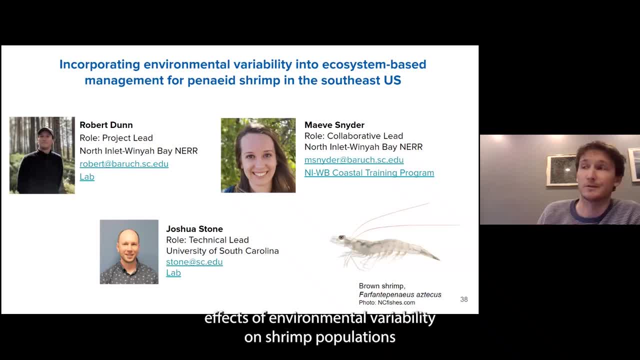 effects of environmental variability on shrimp populations in estuaries of the southeast, namely South Carolina and Georgia. And this is an important issue because shrimp fishery is actually worth multiple million dollars per year and it's experienced highly variable landings over the past two to three decades. So shrimp, just so everyone's on the same page with the sort. of biological background here. shrimp have a multi-phase life cycle that happens on an annual scale, where they spend time in both estuaries and the open ocean. So adults are the target of the fishery. They live and spawn offshore Their larvae then come back inshore. 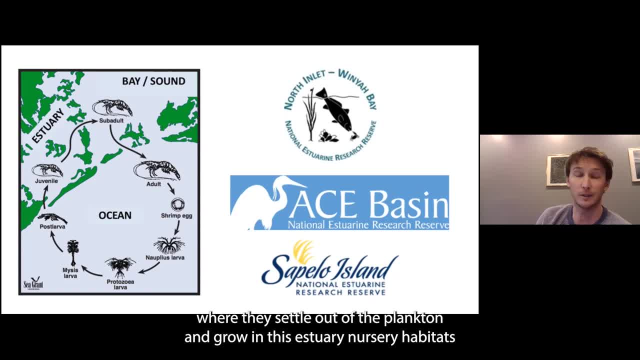 into our estuaries, Where they settle out of the plankton and grow in these estuary nursery habitats before migrating back out through inlets to the coastal ocean. So our project focuses on shrimp populations in three reserves in the southeast: the North Inlet, Winyah Bay near Ace Basin and Sapelo Island. 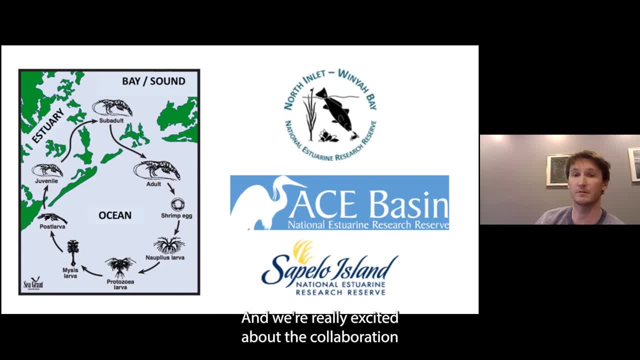 And our project team includes staff from each of those reserves And we're really excited about the collaboration because we're bringing together a diverse group of with expertise that spans different life history stages of shrimp fishery managers from local, from state and regional fishery management agencies. and fishing industry stakeholders, So it's a unique combination of folks. So, in addition to the reserves that I mentioned, we also have team members from South Carolina Department of Natural Resources and the South Atlantic Fishery Management Council, Who's actually the legally mandated entity that manages the regional shrimp fishery. 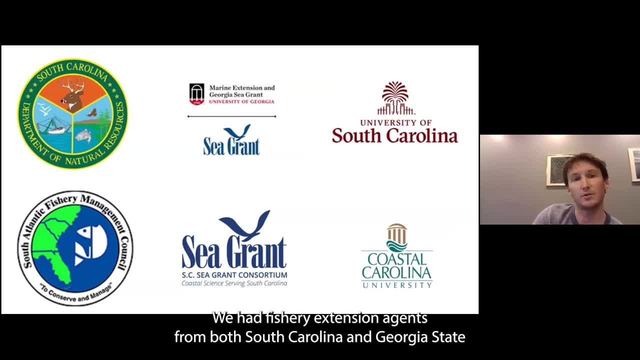 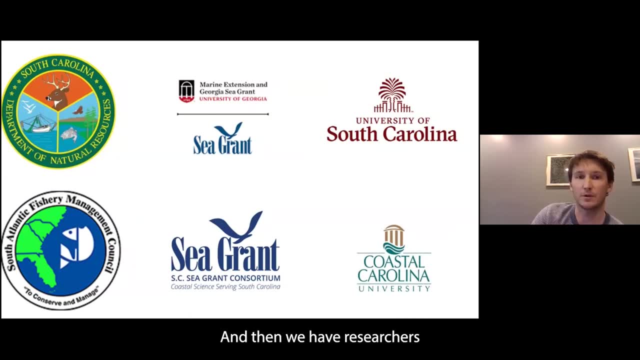 We have fishery extension agents from both South Carolina and Georgia state sea grant organizations who are going to interact with fishing industry folks, And then we have researchers from the University of South Carolina and Coastal Carolina And the management. end users have really already helped shape our project development. 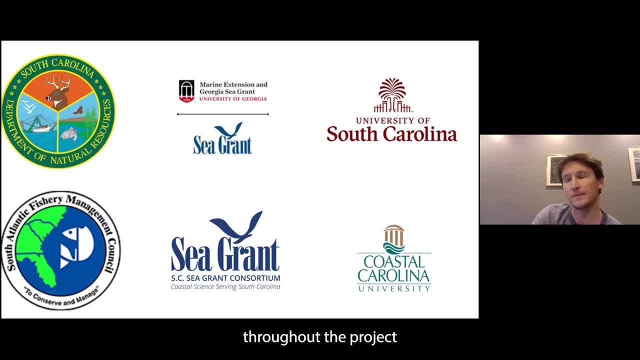 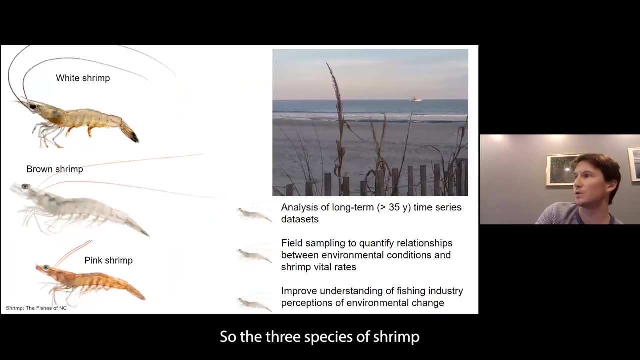 will continue to be involved directly throughout the project through a collaborative iterative process. We'll also be supporting multiple graduate students and numerous undergraduate research interns to work alongside the project team. So the three species of shrimp that will be the focus of our project are white, brown and pinks, all part of the Panaeid family of. 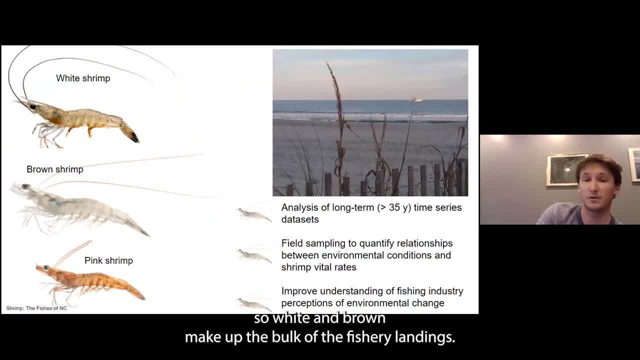 crustaceans. So white and brown make up the bulk of the fishery landings in our two states, South Carolina and Georgia. Brown shrimp start entering estuaries in late spring, stick around through the summer. White shrimp come inshore a bit later and then hang out. 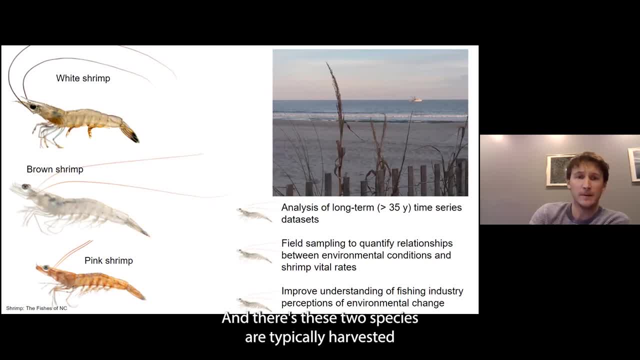 in estuaries through the fall and into the winter, And these two species are typically harvested by shrimp trawlers operating just off shore, like the one in the photo there on the top right. So our project has three main objectives. First, we'll be utilizing numerous long-term 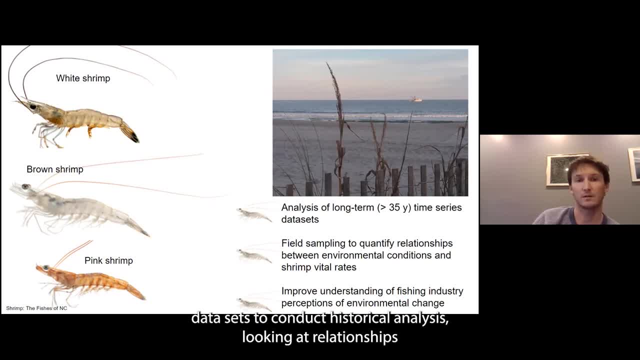 time series data sets to conduct historical analysis looking at relationships between environmental conditions and multiple life stages of shrimp, And so we're excited that our project provides an opportunity to pull together all these unique long-term data sets to gain new insights on the effects of environmental variability on shrimp. 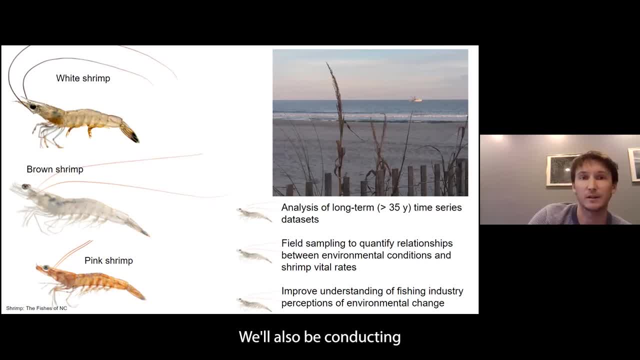 population dynamics. We'll also be conducting two years of field sampling at three swamp stations within each of the three reserves. So at each one of those swamp stations we'll be sampling for three different life stages of shrimp, as well as their benthic prey. So sampling across. 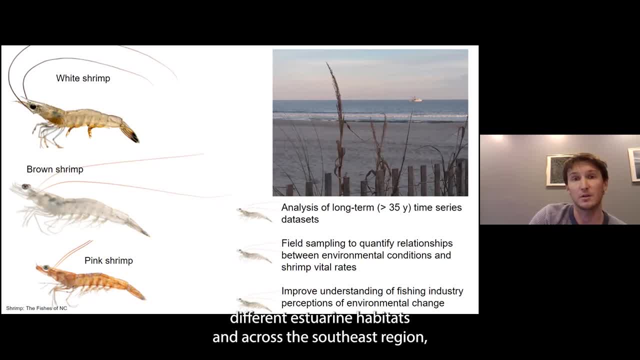 different estuarine habitats and across the southeast region, we think is going to increase the applicability of our results. So we're excited that we're going to be doing that. And then, lastly, we'll be developing relationships with fishing industry stakeholders to better understand their perceptions of environmental change and the impact that. 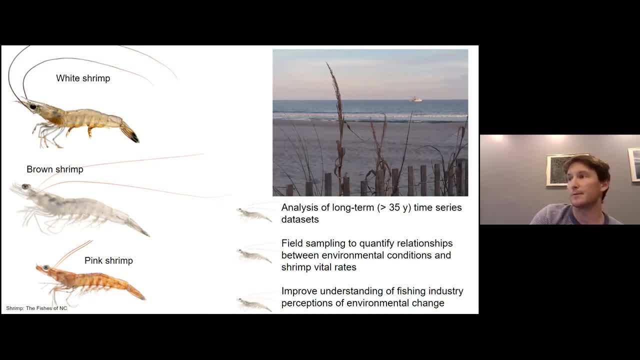 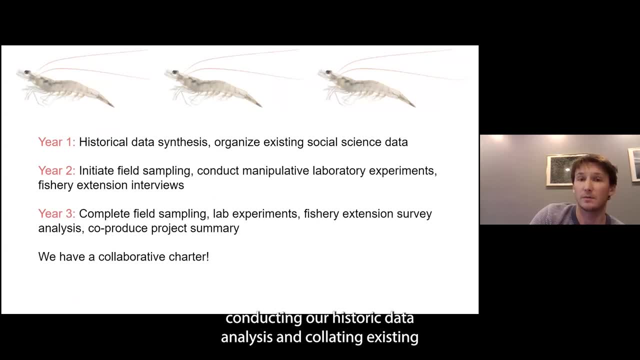 environmental conditions has on the shrimp fishery. So a brief timeline of the project. during year one will be conducting our historic data analysis and collating existing social science data on the Pineda shrimp fishery in our region. During year two, we'll be initiating field sampling which is going to be informed by the historical 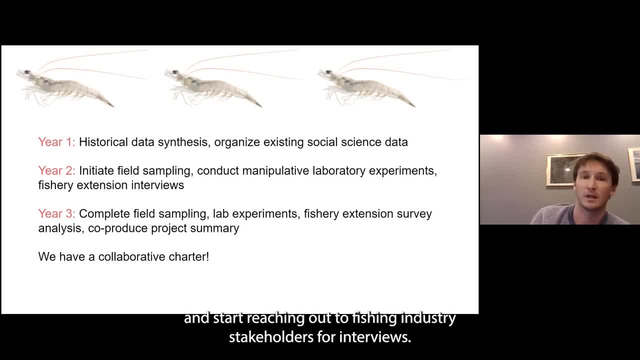 data analysis, conducting some lab experiments, and start reaching out to fishing industry stakeholders for interviews. And then in year three we'll finish field sampling, finish the lab experiments and generate a co-produced project summary document highlighting the main findings from both the social science and the life science side of the project. 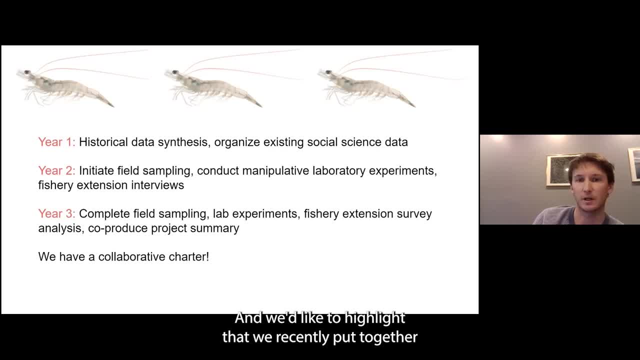 And we'd like to highlight that we recently put together a collaborative charter, which was based on a template that was provided by the Science Collaborative- and maybe Nick or Jane could put that in the chat for us- But we discussed the draft charter with our team. that covers things like roles and responsibilities, how our meetings would be run. 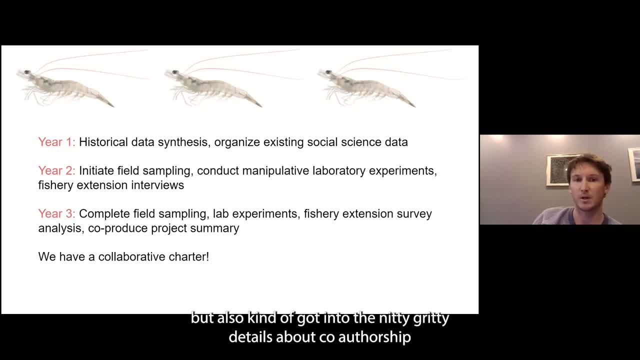 our general principles of collaboration but also kind of got into the nitty-gritty details about co-authorship policies and how we're going to be working with the science and the life science side of the project. So we're going to be working with the science and the life science side of the project.